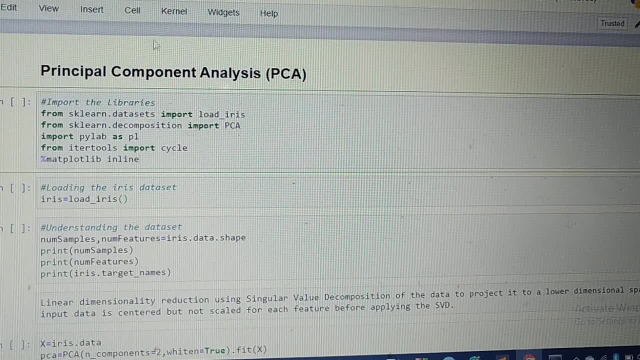 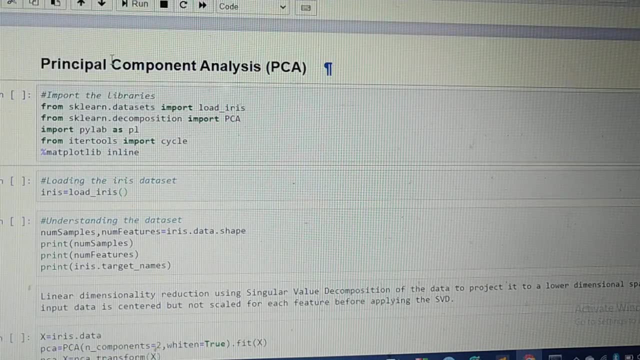 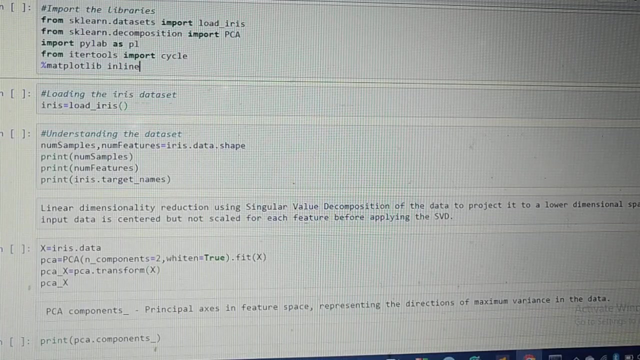 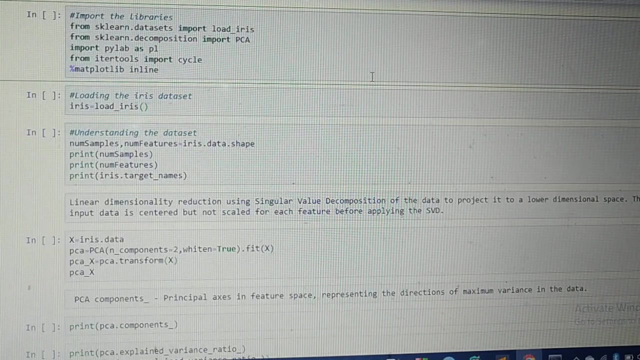 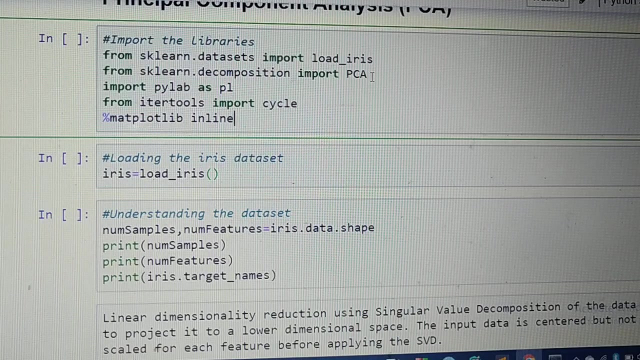 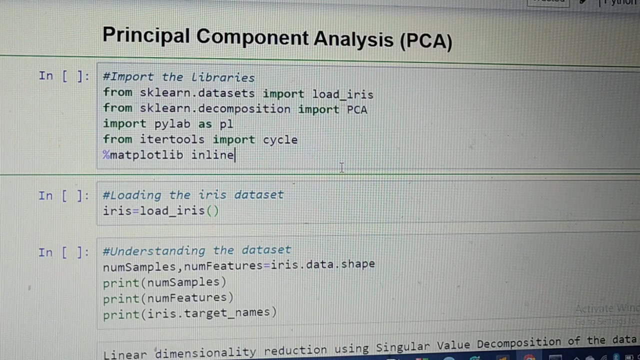 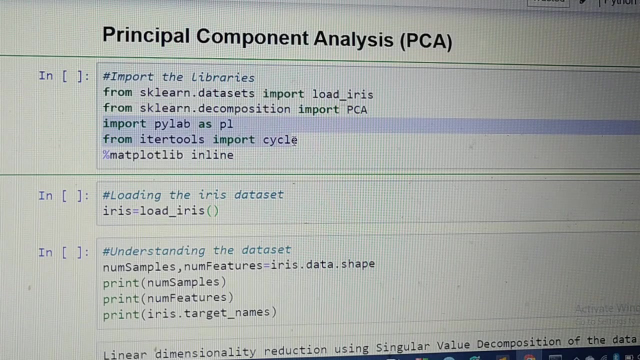 So let's toggle out the header and the toolbar so that we can have more space, and we are going to zoom in, Okay, so first of all we need to import the libraries, like we need to import the data set, and then we have to import from scikit-learndecomposition, we have to import the PCA and then we are going to import some of the libraries for drawing the graph and let's run it. 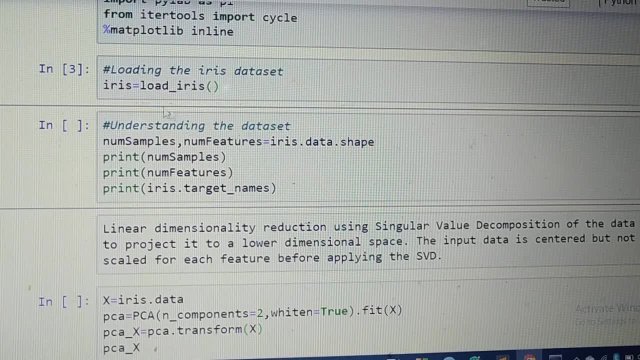 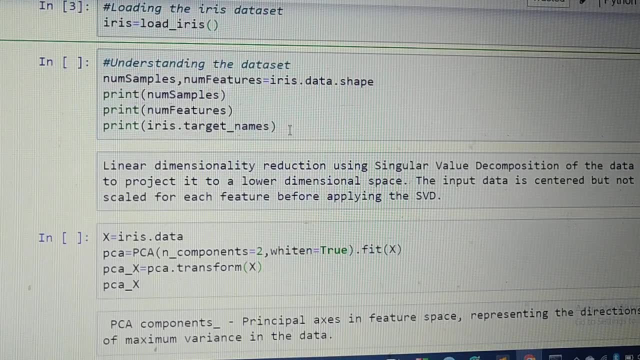 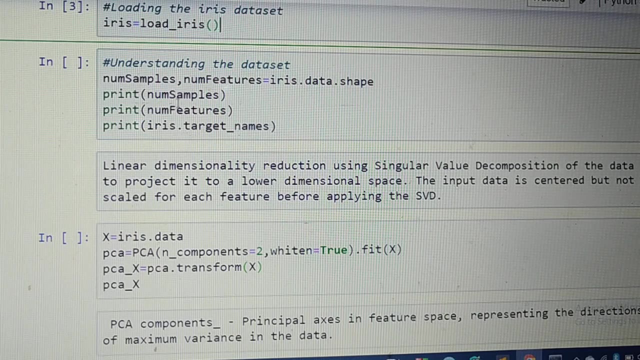 So first of all we are going to load the iris data set. So we will use iris equal to load underscore iris, So the data set is loaded in iris. Next, we will try to understand the data set, like what are the number of samples and what is the features. So num sample and num feature equal to irisdatashape and we are going to print the samples and the features and also we would like to print the target names. 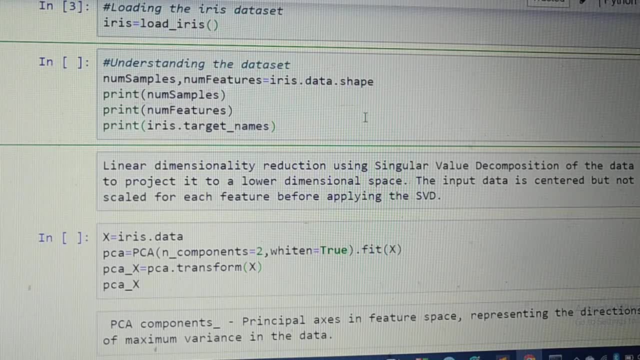 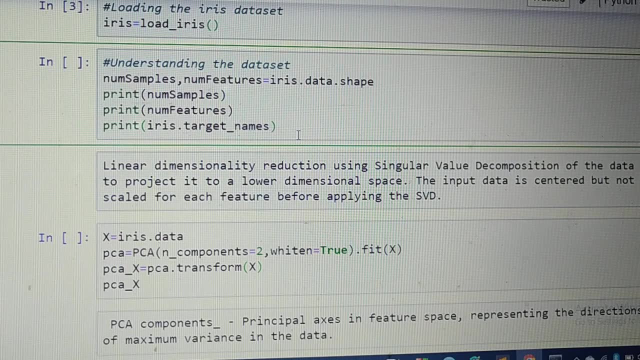 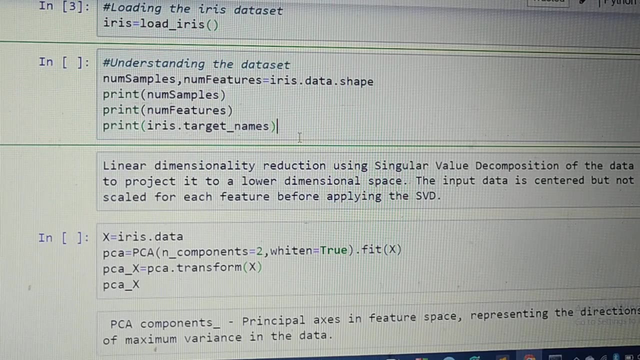 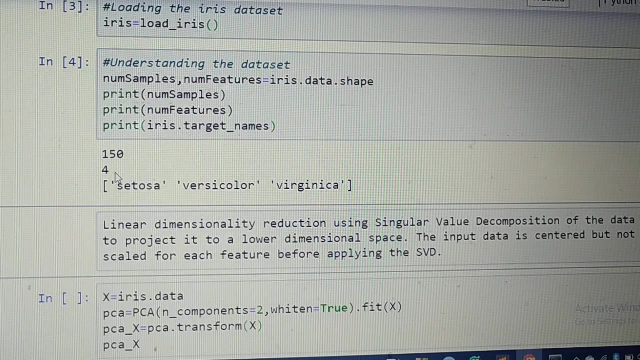 So, basically, if you are very accustomed with the data set, it is like it has got four values and like your sepal width and sepal length, petal width and petal length and then your target names. So there are three target names, let's see. So press shift, enter. So we have a total of 150 samples and four features are there and you have these three target names. 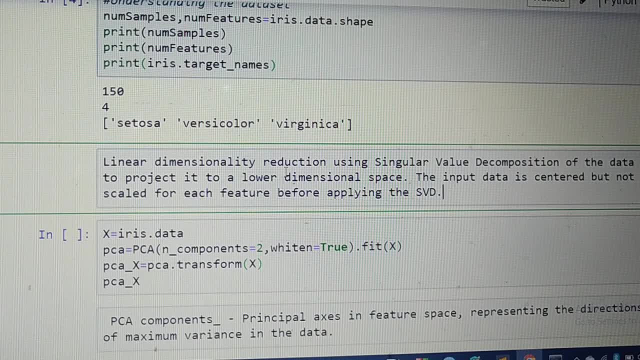 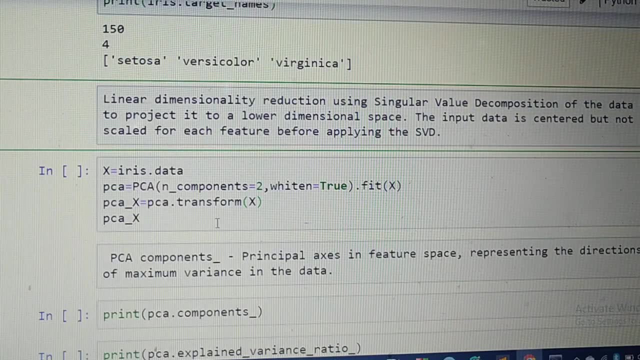 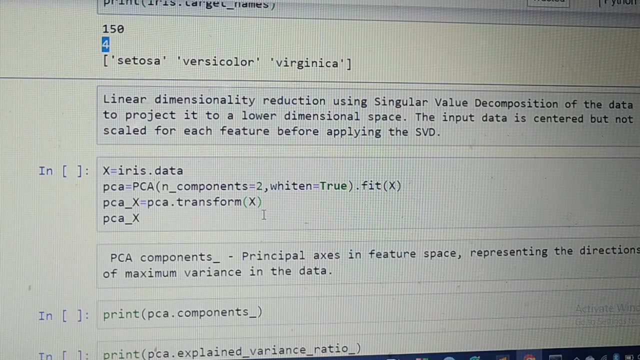 Next we will try to apply, on this data set, your PCA. So what exactly is PCA? It is a linear dimensionality reduction using the SVD of the data to project it to a lower dimension space. So here we have got two features. We want to extract information using lesser number of features. 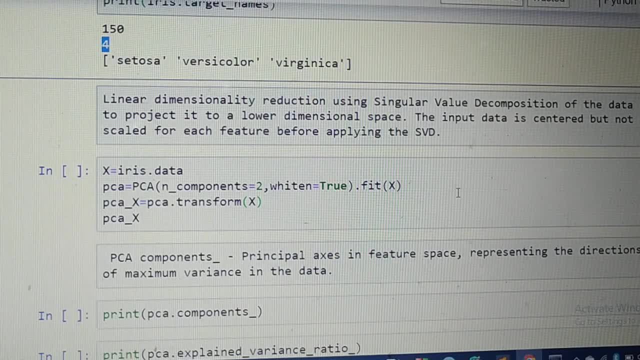 So we will use the PCA algorithm. Let us see how it's being done, And so what we are going to do is that we will. the input data is centered, but not scaled, So first you have to fit your data and then you can scale your data. 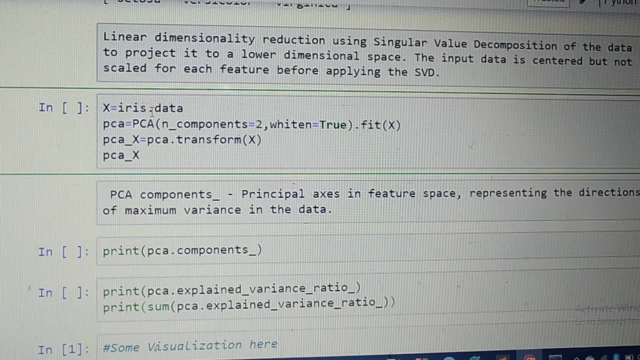 So we have to use, we have to put the data in X, and then PCA equal to PCA, and if you want to know about what exactly is there in PCA And then PCA equal to PCA, and if you want to know about what exactly is there in PCA, there is a variable called PPA. 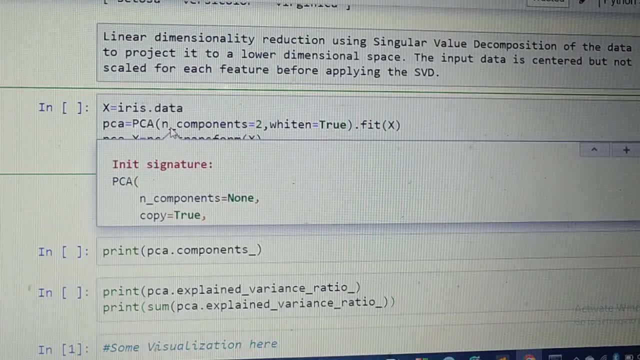 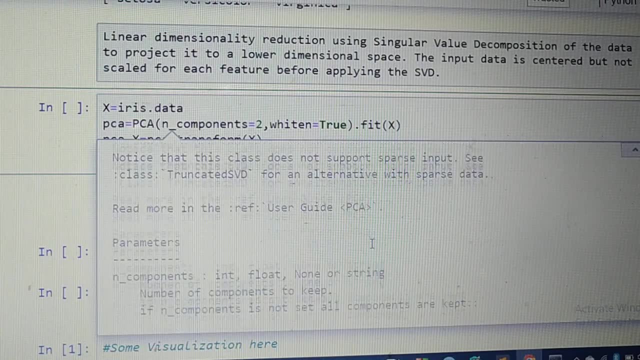 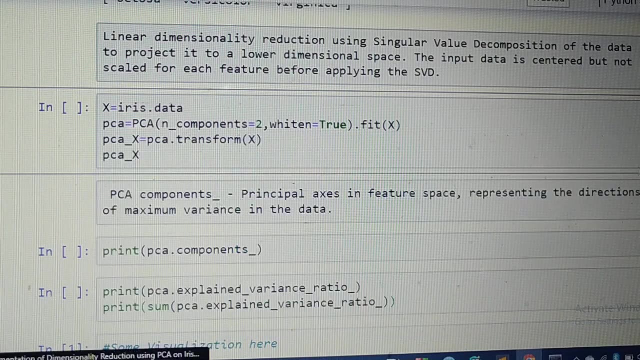 Press shift tab here So you get the entire documentation of PCA. So you will get what is PCA and what are the parameters, what is the meaning of those parameters. It is there So you can have a walk through that. So what we are doing is that we are taking n components equal to 2. That means out of 4 features, 4 components will take 2.. If you are not mentioning the number of components, it will take all the components by default. 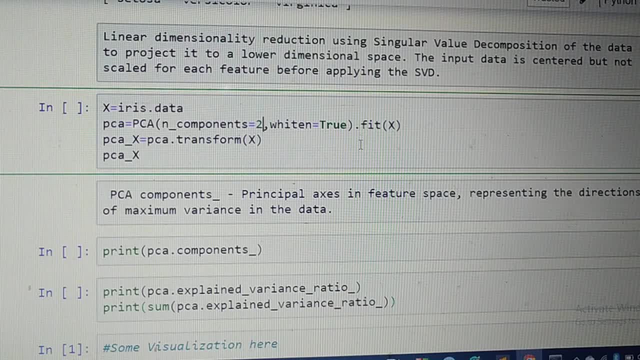 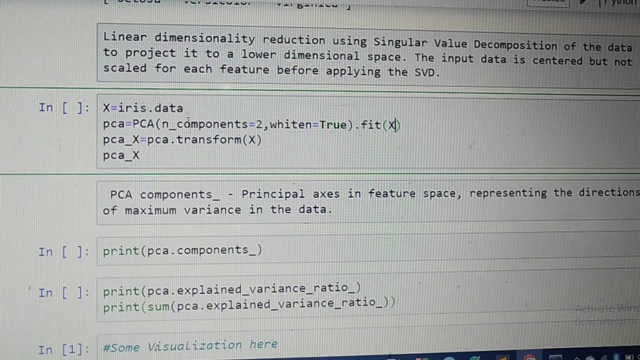 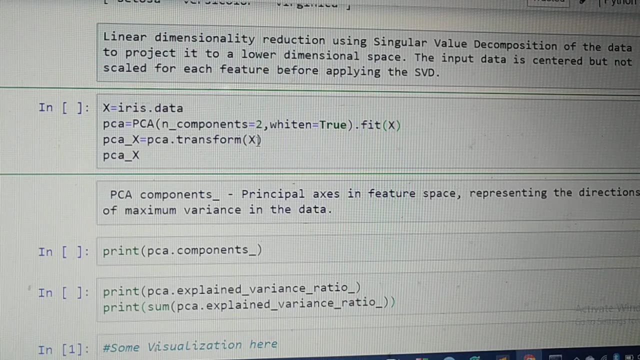 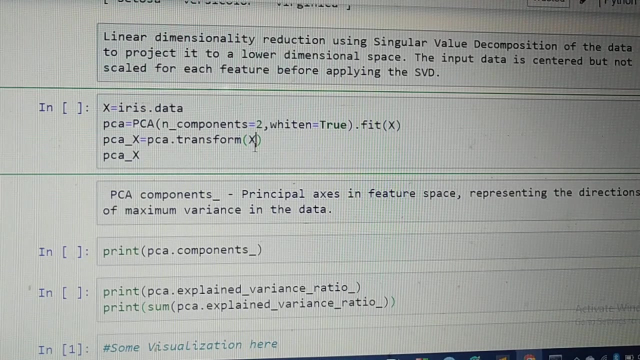 Yn equal to 2, true, so that your prediction will be better in the estimate Fit x. So we are going to fit our data. Next, PCA underscore x is going to have your model, which is transformed. So we apply the PCA on your data set now. So let's run it So. 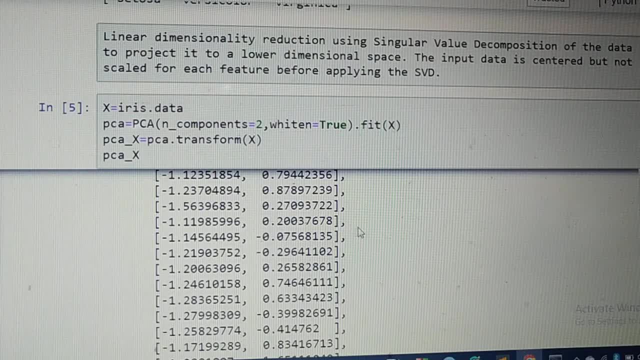 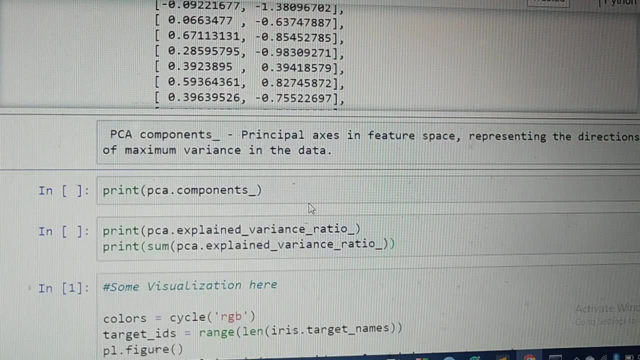 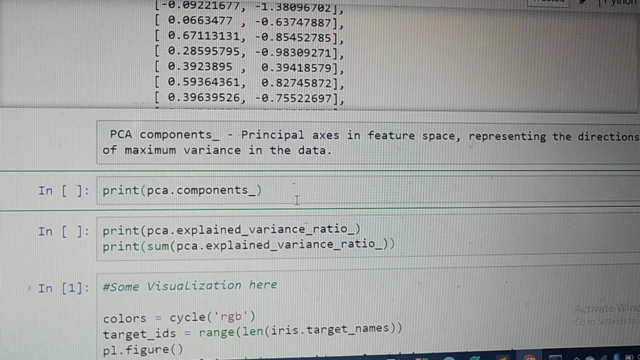 here now you can see only two features, two components here. Next we would like to see what is the principal component attribute. So principal axis means here we are using, you know, two. we require two components. that means you have two orthogonal division on your features. So in the PCA component you will get the representation of your maximum. 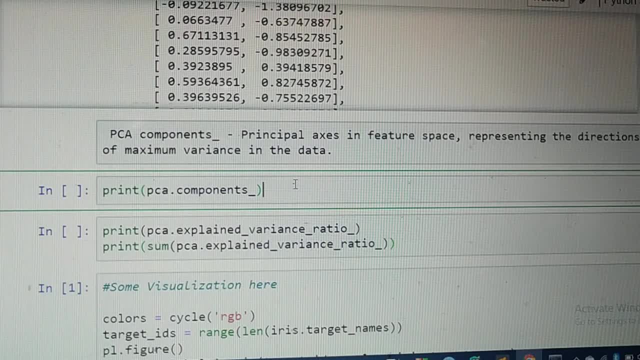 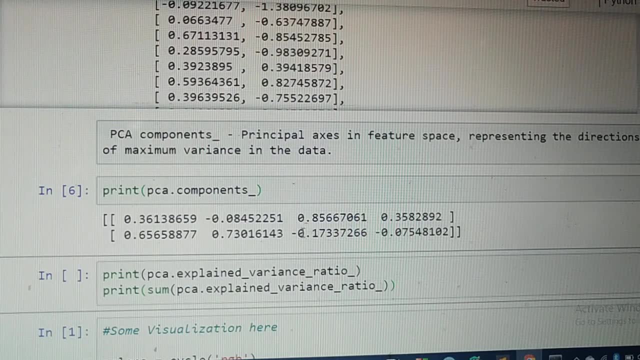 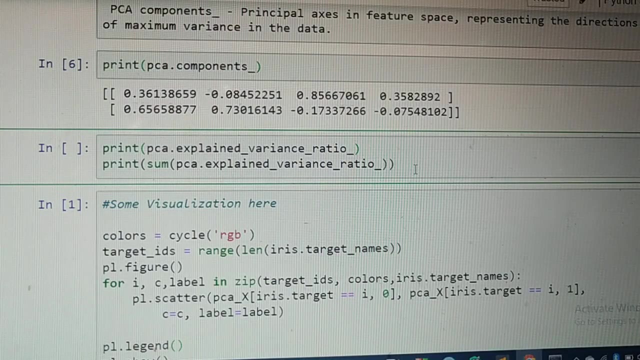 variance in the data. So here, when you want to print PCA dot components underscore, you got the value of your PCA component underscore and then we would like to find out like, since we have taken only two components, what is the amount of variation of your data set is? 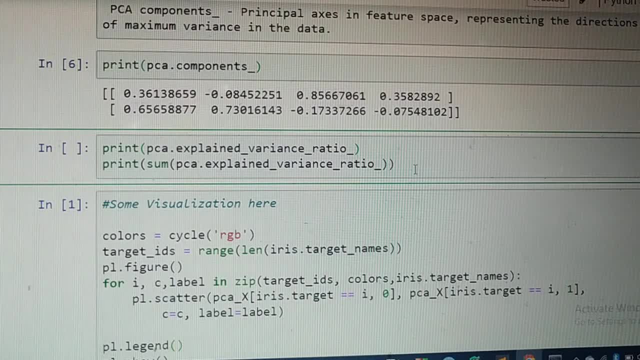 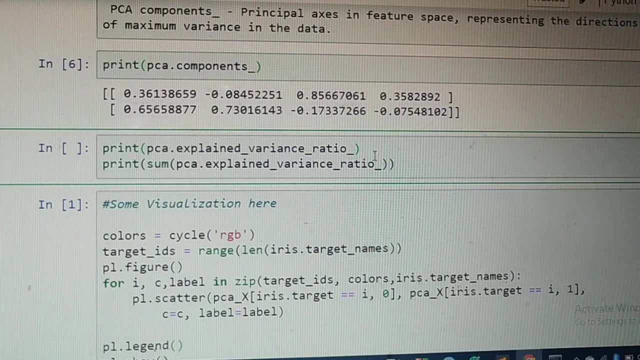 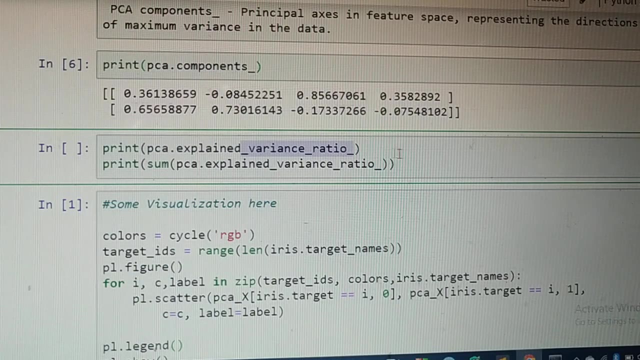 explained by having only the two components. So we will take PCA, dot explained underscore, variance, underscore, ratio, underscore. So this is going to give you the ratio, your variance of the first principal component, the second principal component and this. then you can find the sum and you can find out how much. 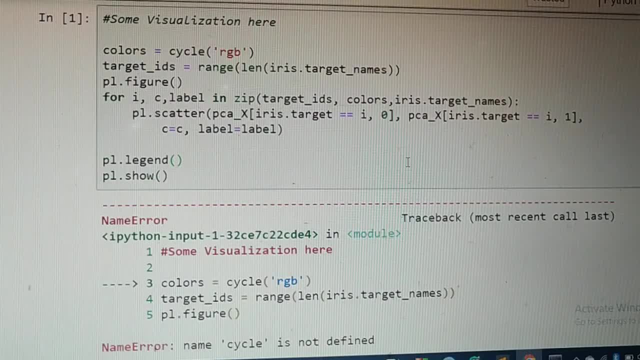 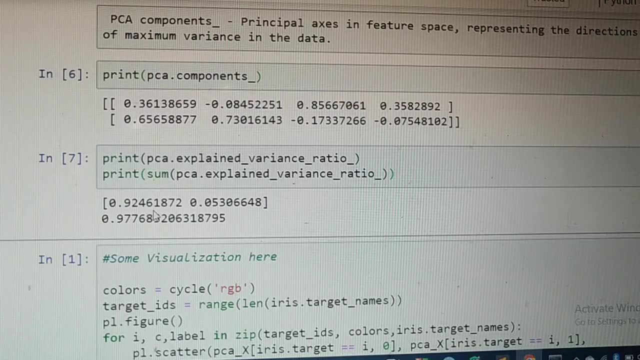 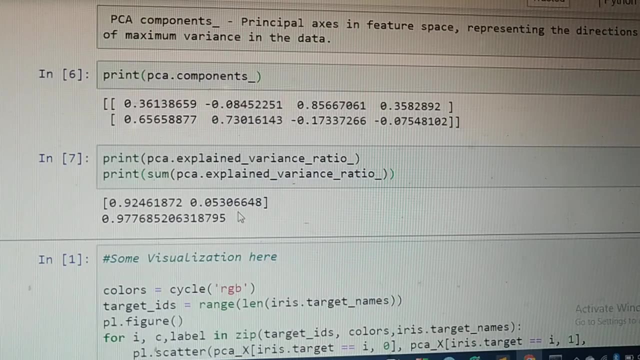 variance you are getting after applying the pca. so we can find out. the first principal component is giving 92.46 percent. that is very good. and the second principal component is giving, you know, 5.3031. you can take it and when you sum this you are going to get overall. 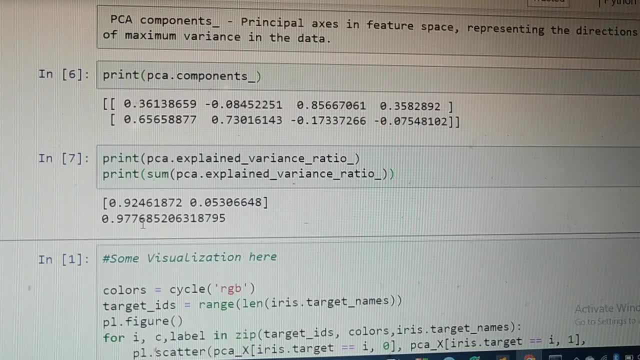 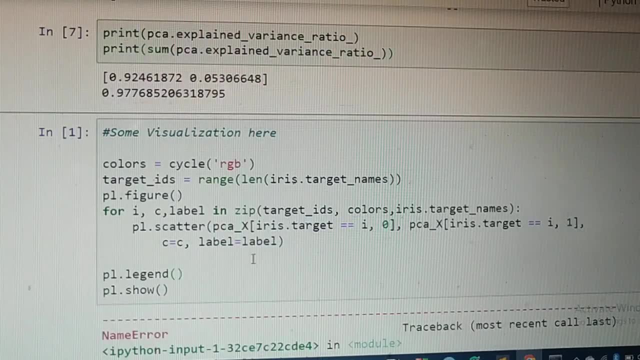 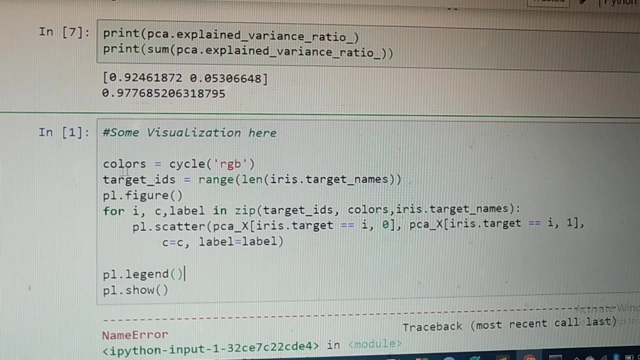 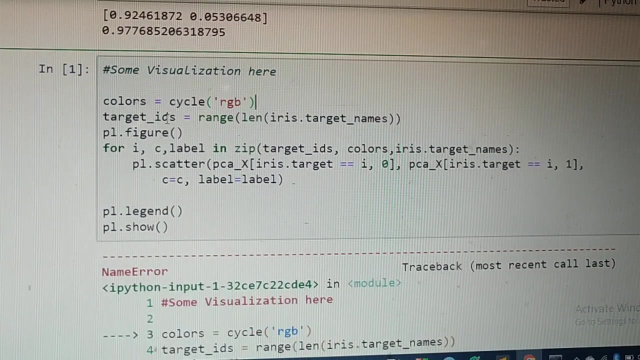 variance in your data set of 97 percent. that means that's a pretty good amount. you can easily explain your data set. now let's visualize your information that you have. so what are we going to do is that we'll take colors equal to the cycle- rgb color- and your target ids is going to be: 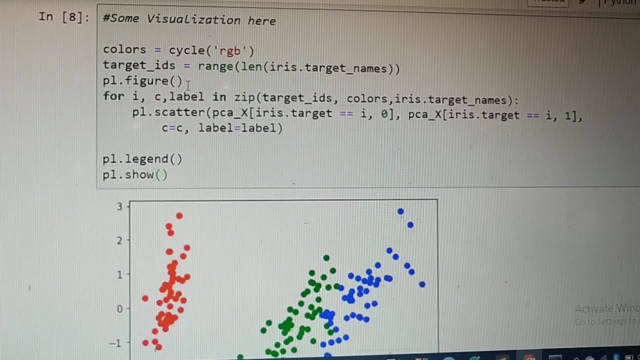 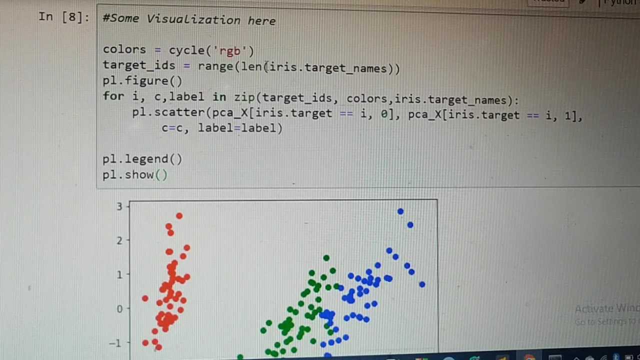 let's run this first. okay, you. so your target ids will be your range of length of iris dot target underscore name. so iris dot target underscore name has three names, so the length will be three and range- if you apply range, it will be 0, 1, 2. so that is the value you are going to get in your target ids. then you are. 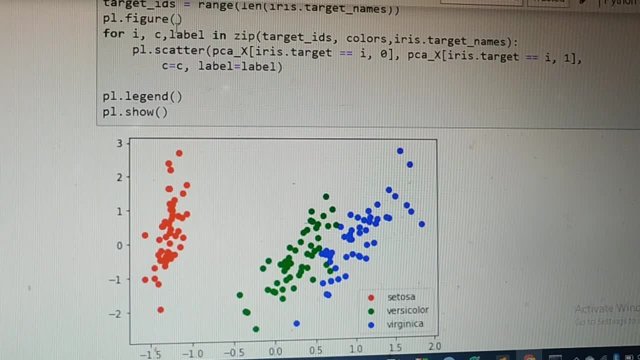 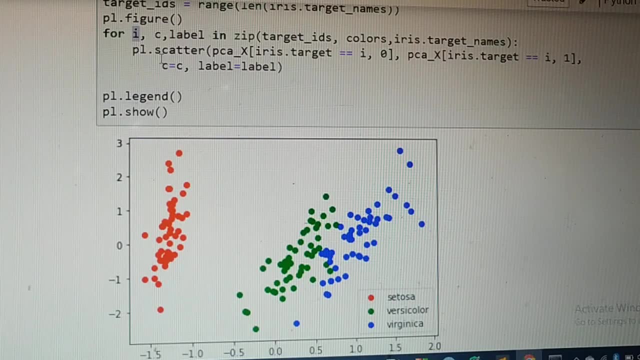 going to. uh, you know you want to go draw a figure for i, so you have your for i. this will be a index. you know the value variable and c is the color and l is the level in zip target id. so what are you going to have in your target ids? you're going to have first, you're going to have 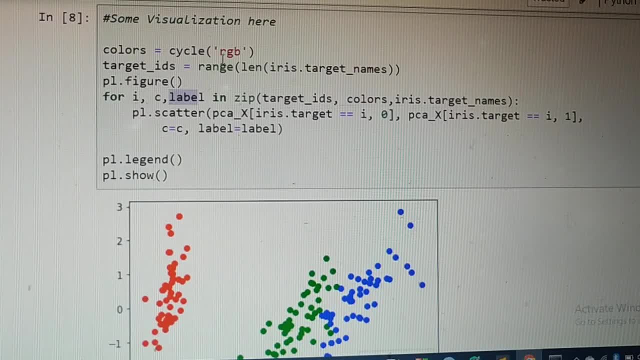 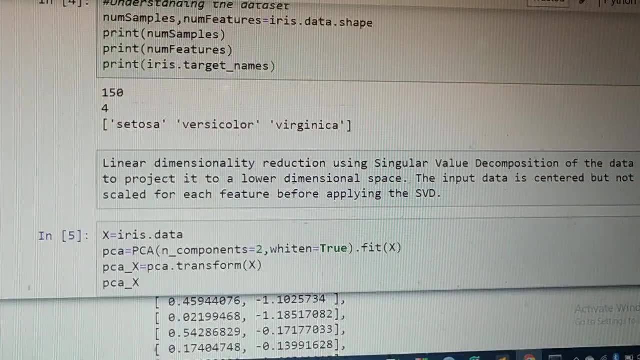 zero. zero will be zipped with red, and this is your first name. that is your uh. first target name is cetosa. okay, so then you have versicolor and then you're going to see what color is. this is what color. so in this we have hart onwards and backwards. we will have 150 hundred. so this will be values. eso is.